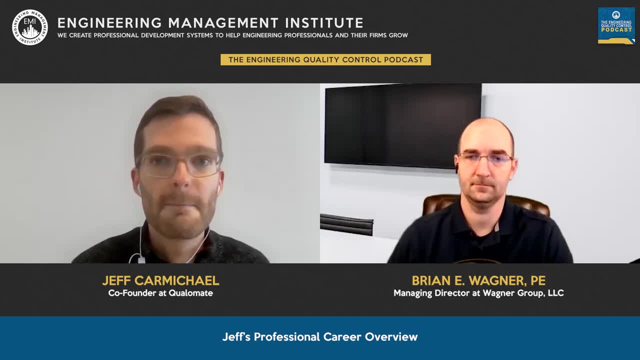 in construction and civil engineering. So yeah, after about three years down there, I moved home to Canada and started building a startup called Qualimate, And essentially what we do is automatically extract data from construction documents- like, specifically, like inspection reports and test reports- And then we map that data to a physical 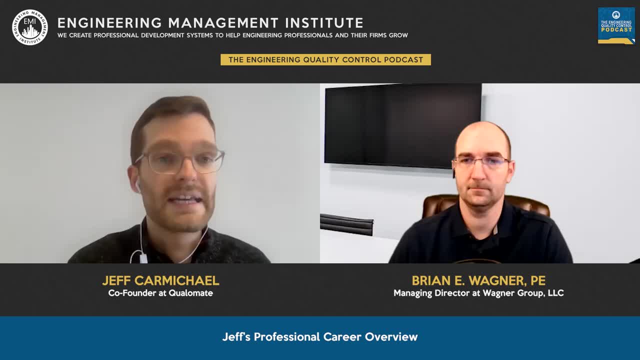 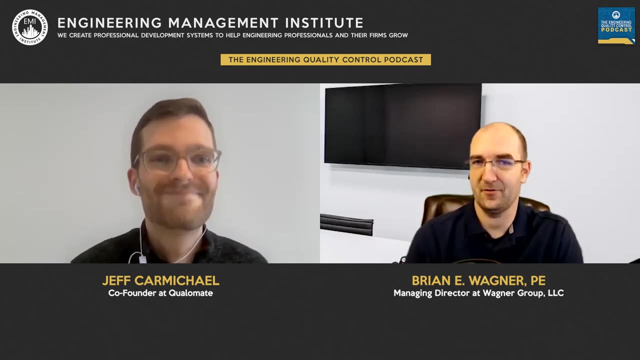 location on your project And it's kind of like an interactive map that you can use to keep eyes on your quality program and reduce the risks that come along with not knowing exactly what's going on And that's somebody that's. You don't have to read every word of every report to catch those little things right. 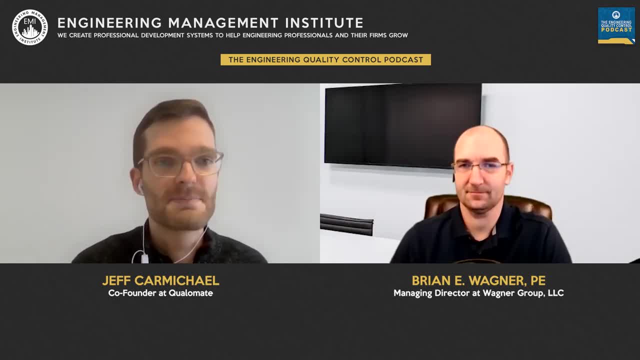 Exactly. Yeah, It's very visual, So it's all tied to your specification. So if it passes the spec, then it turns green, If not it's red. then you've got some more work to do, So I'm kind of doing all. 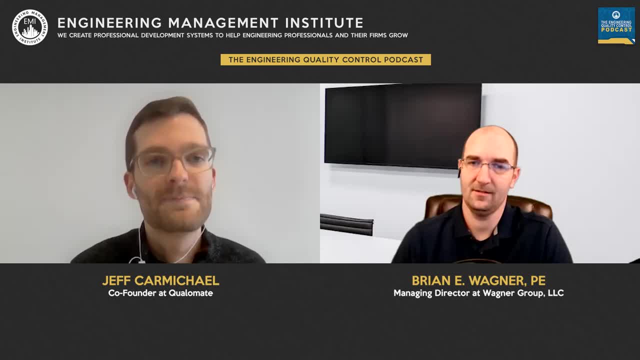 the software development for that, as well as the kind of business side as well. Okay, So from your experience on the infrastructure projects, where did you see like quality management challenges in that experience that you had? Yeah, I think the biggest thing was the planning of the execution. So most people in the business 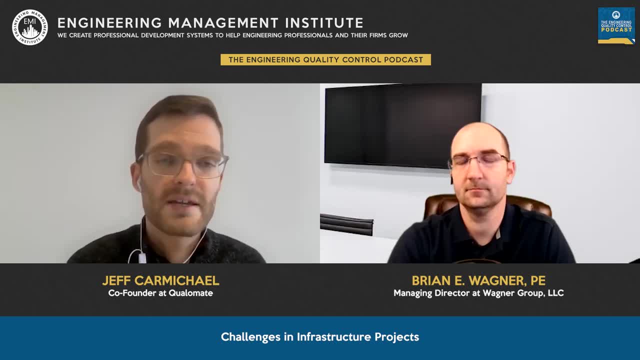 will do a really good job on. They're having inspection and test plans and those sorts of documents. But when it comes to the actual in the field, making sure everybody's on the same page, we found that to be a bit of a struggle, which is sort of where I'm coming from things. 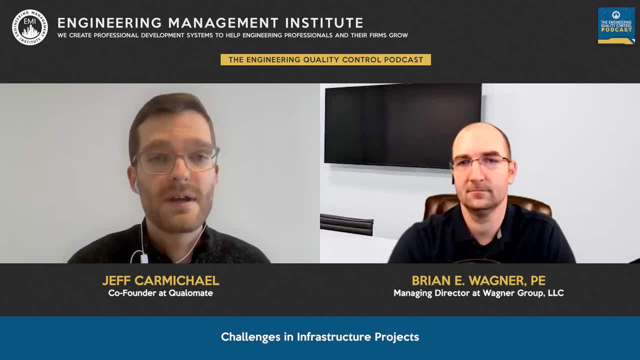 So yeah, for example, having your local Yeah lots well-defined and planned out ahead of time. So you know we need this many tests in this area, but also making sure everybody on the project knows where those lots are. And so there's. 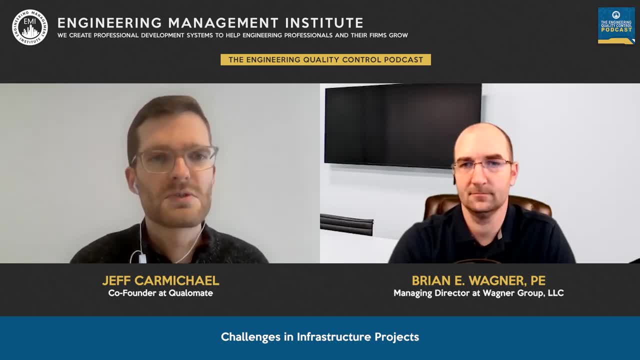 no double testing or overlaps and just those sorts of chaotic things that can happen if you don't plan out that actual execution of your quality plan, Because planning it before pre-construction is pretty easy. You make the documents and hand them out to the field. 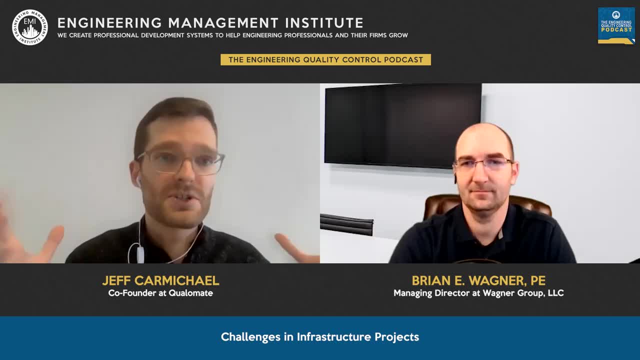 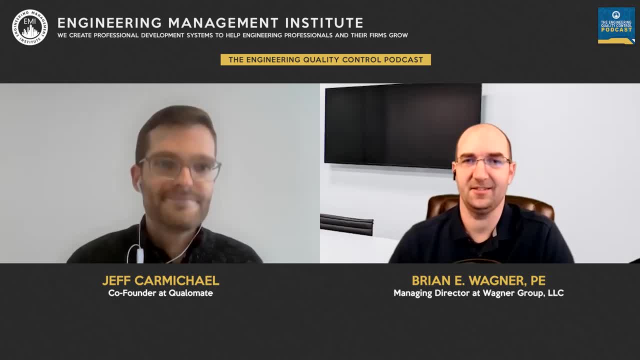 Right, Okay, When you start talking hundreds of thousands of feet and distances and I can understand where it starts to get confusing- Doing different things at different phases and different people and different individuals and different companies. It's like the game of. 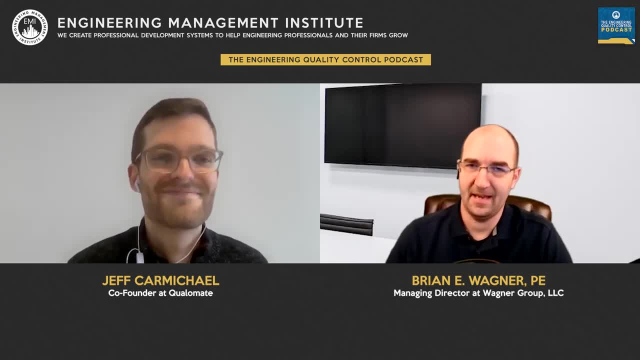 telephone that we all played when we were in elementary school, The message can adversely change Exactly. yeah, Yeah, you've got so many different teams that might be doing the exact same thing, but doing it in totally different ways, just in different areas. um so, yeah, yeah, that was. that was definitely a. 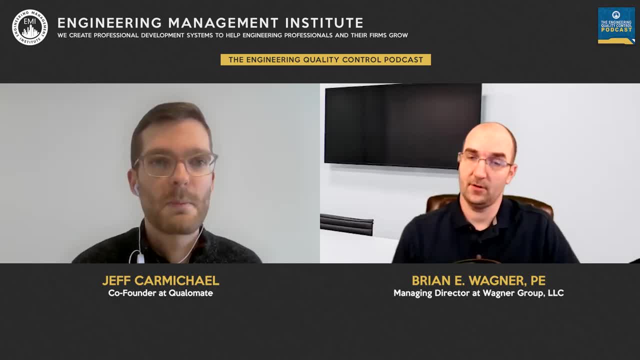 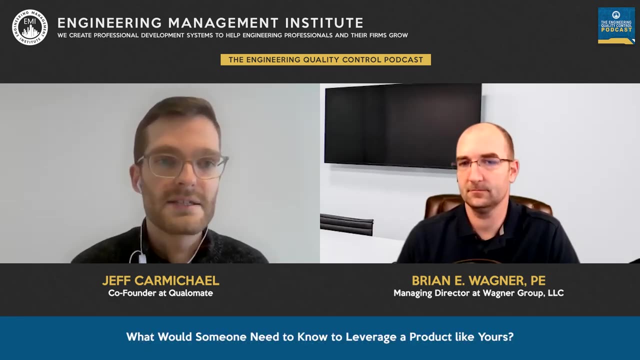 struggle. so if somebody was to like use a product like yours, do you have to know coding or like what? what would somebody need to know in order to kind of leverage a product like yours? very little in terms of uh, of that it's. it's designed to kind of incorporate your existing. 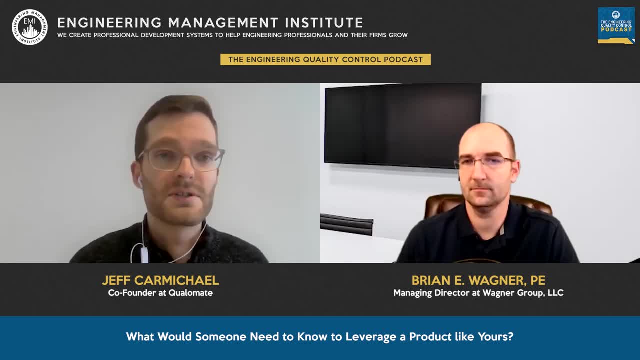 workflows, so it's all based around emails, so you can just email your documents to the system, so that that part is is pretty easy. and then creating the lots themselves is kind of the only tricky part. but you can import them from if you've got your cad drawings like a dwg file and things like. 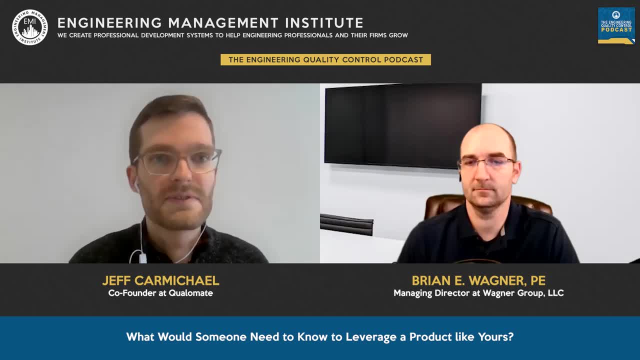 that. but then you can, um, you can import them from your cloud and start talking to a consultant and start making your own advanced software and um, and so that's kind of the way I'd like to say you can also kind of draw them on on the map. so it's very, uh, designed to be very like user-friendly. 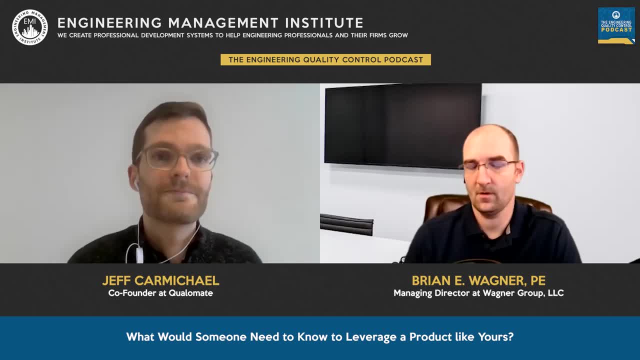 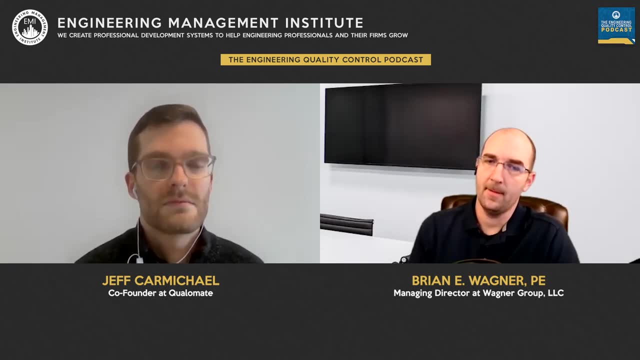 and a shallow learning curve, essentially okay. so we've talked a lot about um, the engineering and construction documents on the show, but you've kind of developed the software. so it's a little bit different in your approach to, probably, quality management. but i think that, like i say, with 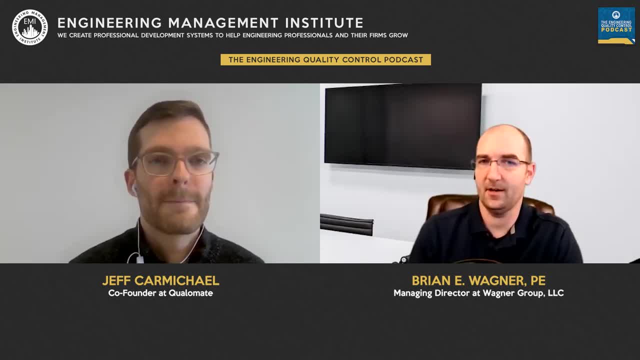 everything when it comes to quality and it's learning and leveraging those experiences and those insights and nuggets of information from across the spectrum of what we do as engineers. so do you have any like advice on, or can you shed some light, i should say on, how you manage the? 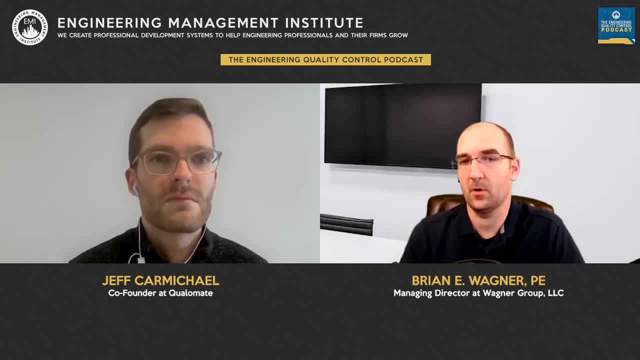 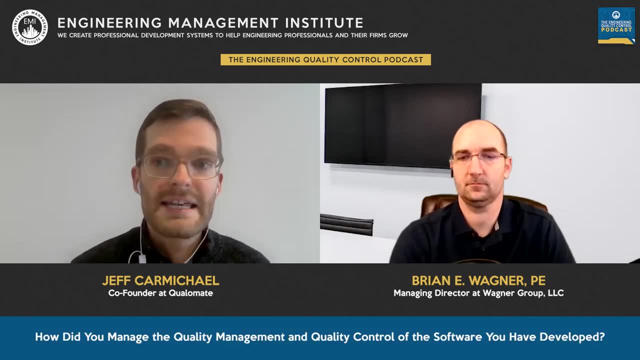 quality management and the quality control of the software when you were working on it and developing it? yeah, yeah, it's a great question. um, so it's, it's. it's relatively easy because, in terms of, from my perspective it's, i'm the sole developer right now, so it's. 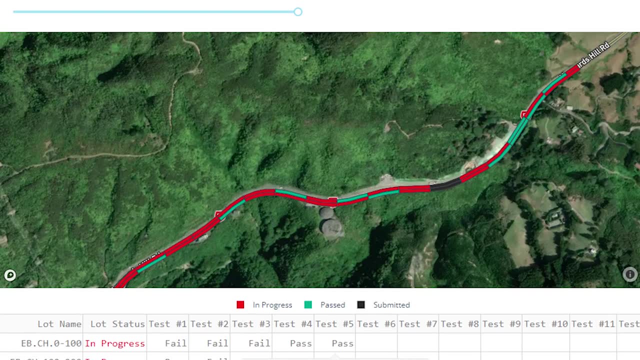 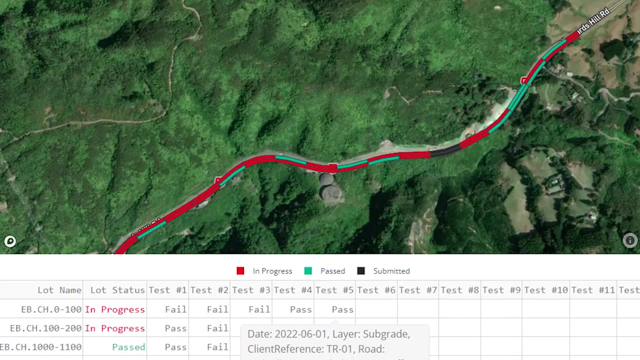 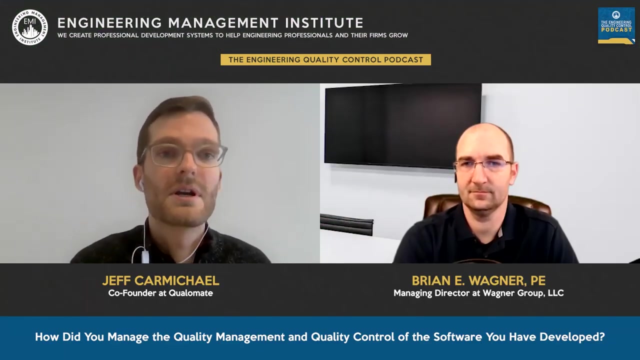 it's um a lot of, just you know, uh testing it out um on my, so i build it on um my local computer and running things there um, and then just going through that entire workflow of you know, creating, setting up a new project on my computer um and doing the whole thing um before i actually uh. 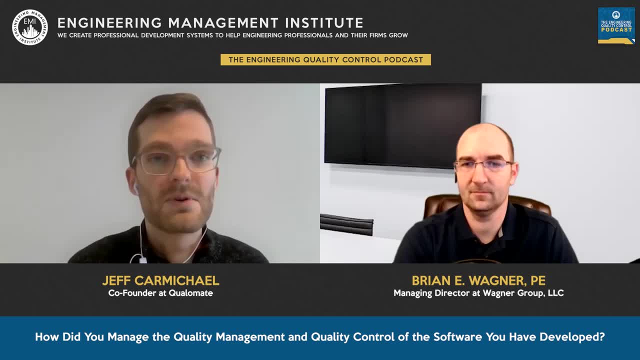 you know, push it to to production so that, so that people uh can use it. so there's, there's that aspect of it as well. but then, even kind of before it gets to the point where it's like, oh, i'm going to do this, to that point there's a lot of um outside of those kind of main files that that build the. 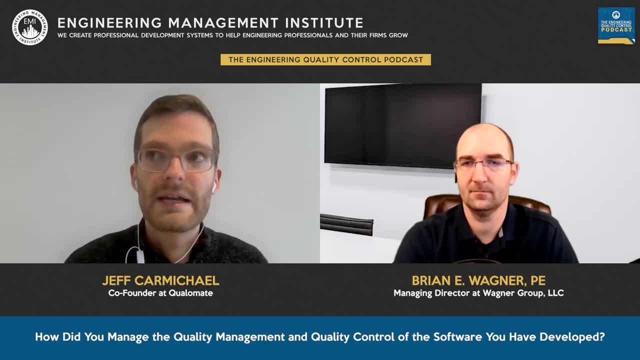 program, um doing kind of off the side in like in a different uh um kind of like a prototyping type environment, um, you know, setting up inputs, that that the system will process, which is kind of more standardized um proper software development qa type approach. um, so, yeah, yeah, having that separate prototype environment for just one small aspect of the 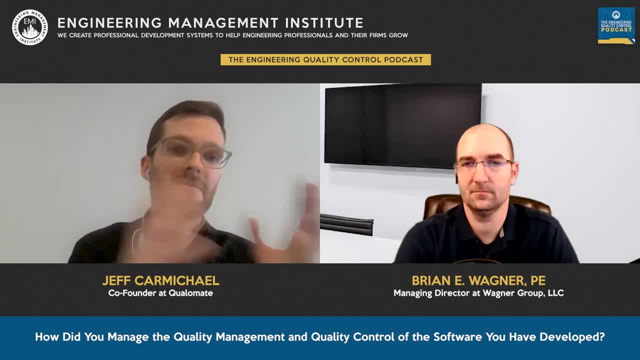 system that i'm building and then making sure that system works, and then you kind of incorporate it with the whole thing and then do the full tests of of uh how it goes. so that's been an interesting kind of learning experience for me, coming from, you know, civil engineering background where quality is. 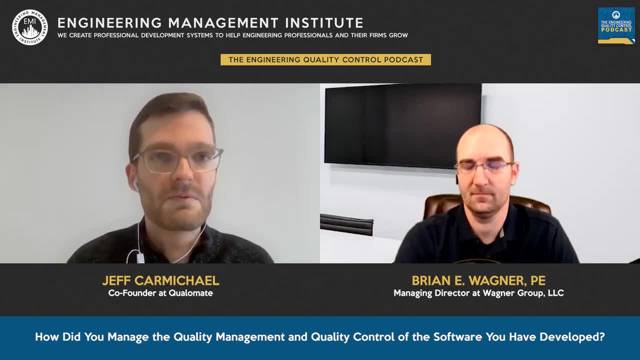 you know fairly, you know standardized and well understood and laid out, but then the quality from software development perspective is is very different and and requires kind of different procedures. that is in interesting learning, and then you know learning all the best practices from from that side of things as well. it's been cool. yeah, because 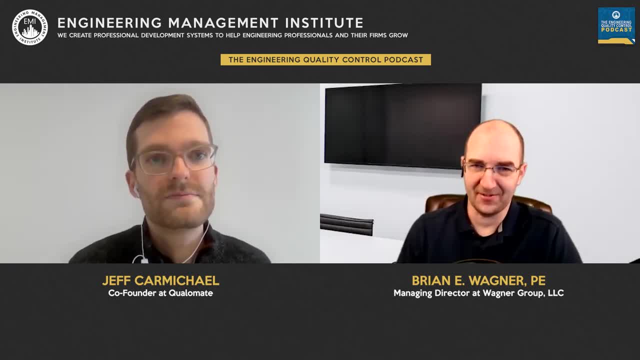 ultimately somebody's. when you bring people in to help you on your software, they need to be able to follow it and not break it right. exactly, yeah, yeah. so having everything kind of laid out and organized is very important and it goes back to those standard practices: consistency, 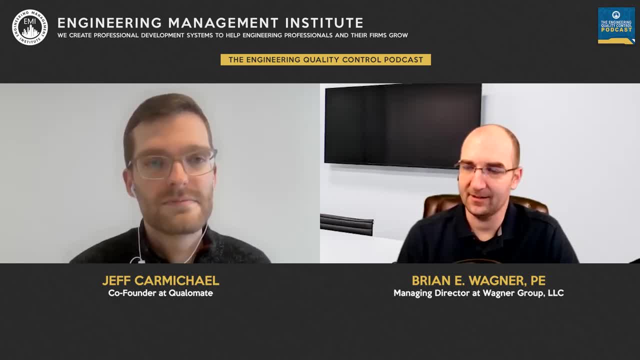 that, that you're kind of going. i mean, i think that's about like i think about the evolution of cell phones over the years and i always said- and i see it with cad too- like the, the technology that autocad has or civil 3d has, within a version or two, microstation and and inroads is coming. 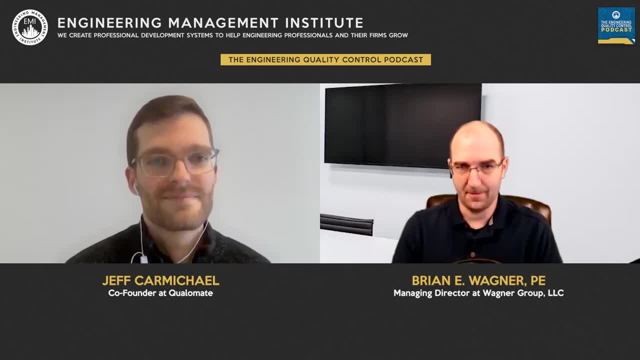 out with that from bentley or vice versa. like it's just, they're building on each other's technology and those ideas and those concepts and with that, i'm sure- as you're you know- you're going to be able to create different or improve things and add more features and things. 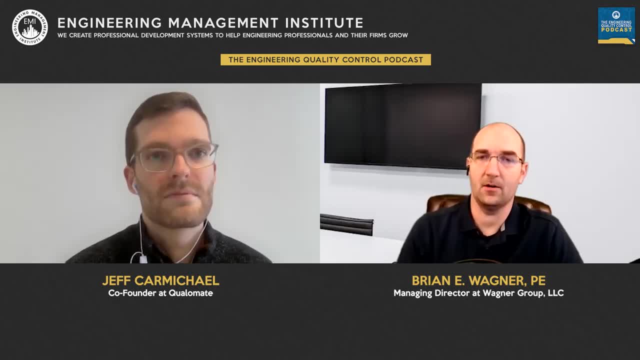 like that. that quality that you're doing in your early steps is vital to that long-term success. yeah, absolutely, because there's, you know, kind of with any product really, you know you build your core set of features and then, as soon as people start using it's like, hey, can it do this and can. 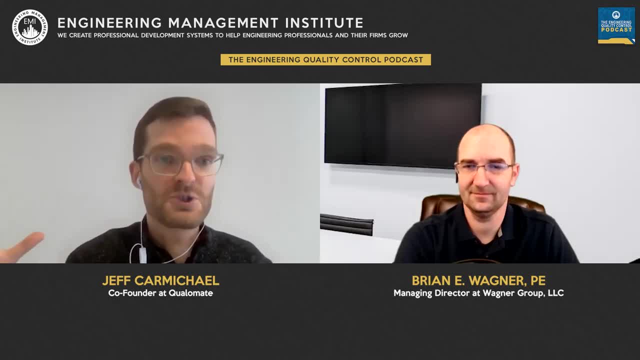 it do this, so you start adding those things in. so, really, your code base just kind of grows extremely, extremely quickly. um, so one of the great things about development is that, uh, it's quite easy to do things repeat like things that you have to do multiple times. it's very easy to to not duplicate yourself, right? so you kind of define a function. that does a certain thing, and then you can call that same function from different aspects of the app. so it's, you know, querying the database. you only have to write that once um across your different you know features, assuming it's the same data that you're looking for, um, but yeah. 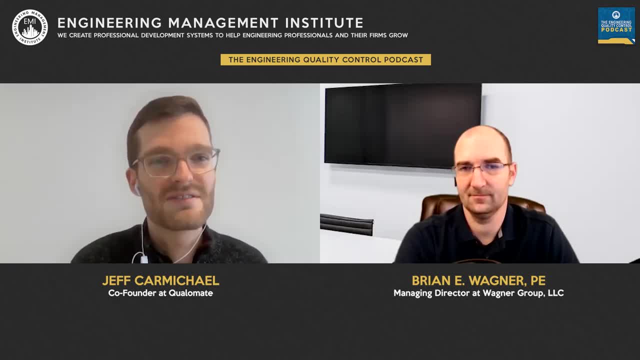 it's nice that that we kind of don't get, especially in construction, like some in some aspects you do, if you're building a building and all the rooms are the same and it's kind of the same same idea. that kind of goes to that like pre-fabrication almost, um, but in my background in the kind of 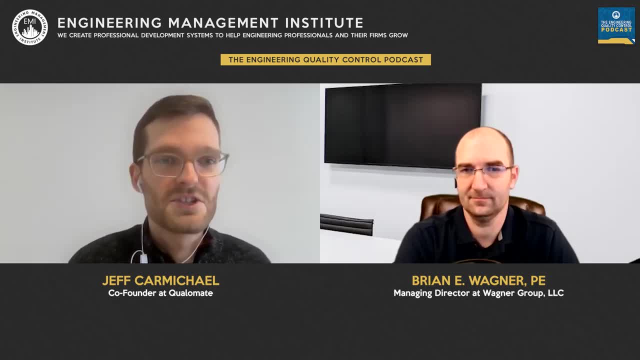 civil space, civil construction is there's not much modularity when it comes to building a road, if you're digging through the dirt, it's kind of different every time. right, i mean, that's where you you skip that. save as issue that a lot of construction and the civil engineering problem. 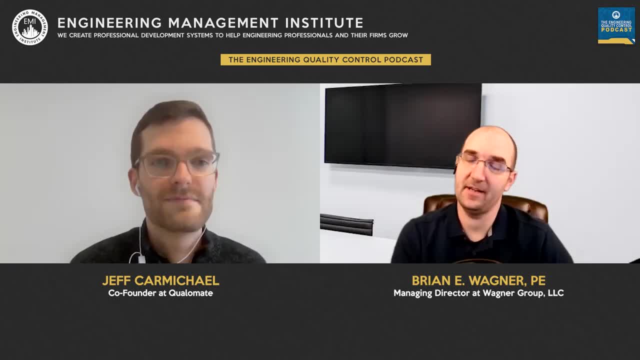 is when you take it from another job or take it from another and then you only edit part of it or change portions of it. you're you're saying that if you call back to that original and that main one, then you don't have to worry about it being wrong or being save as per se. that your structure, your 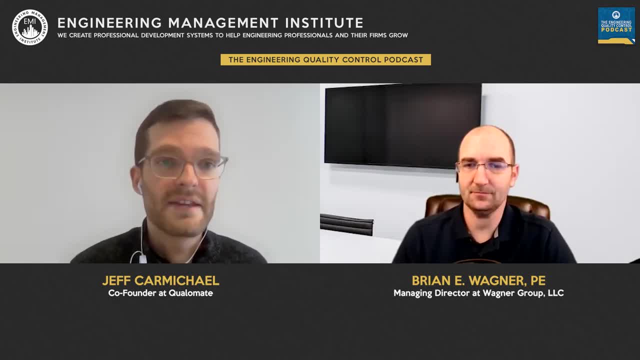 piles and your silos correctly, exactly, yeah, and that's one of the benefits of kind of this sort of digital transformation that's happening in the construction industry, where a lot of the players are using kind of similar softwares- uh, that do kind of a lot more um. so if you've got some workflows, 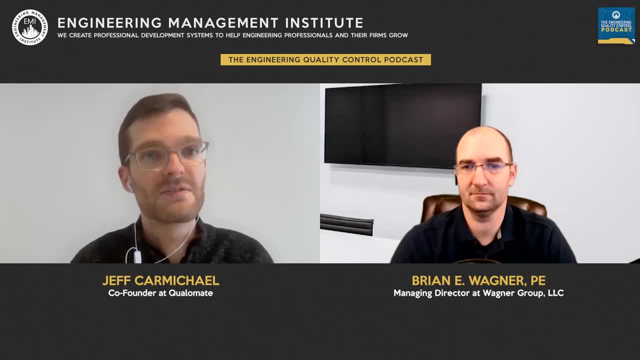 like, if you're to set up a workflow in your software for this project, then you can easily copy and paste that across all the different uh projects that you might have, so you automatically get those kind of best practices that you've established. that's, you know. the same as calling a 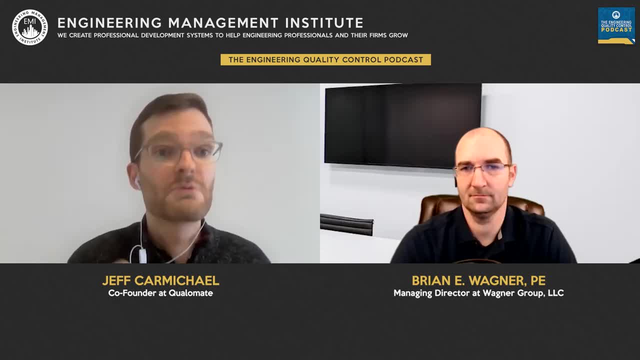 function in the software program. um, that you, it's just the repeatability is it's really gonna be key, especially like with, you know, workforce shortages and all these kind of problems with people retiring and just passing that knowledge around is, um, something that's sort of learned over the course of an. 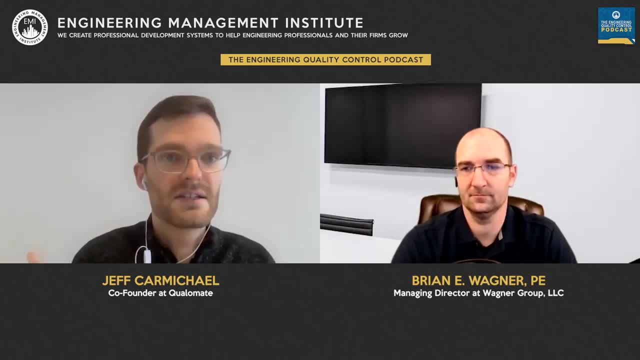 entire career. being able to transfer that very quickly to the next generation, where you don't necessarily have a lot of overlap is, is going to be really important. so i think software is going to play a big role in that from from all aspects of civil engineering and construction. so for for. 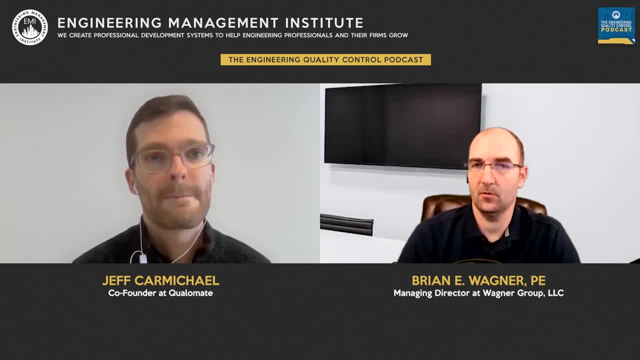 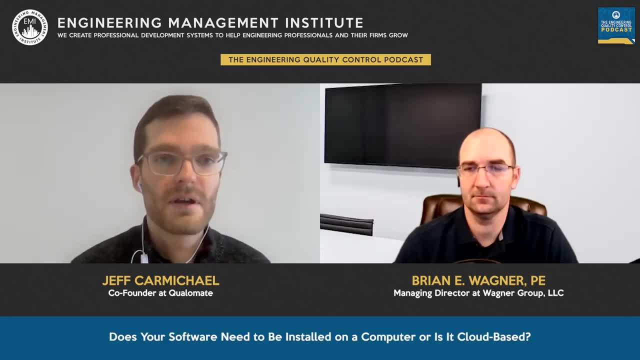 yeah, so it's all all cloud based. it runs on amazon web services, which is just not coming from a software background- software education myself- um is is kind of uh really amazing once you start to to learn about those sorts of offerings from those major cloud providers. um, there's just so many. 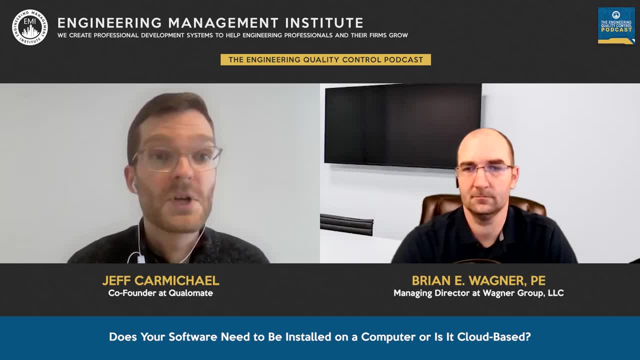 features and they make it so easy to to, um, you know, set up a software company, really like once you know what you're doing. um, and compared to how it used to be, say, 20 or 30 years ago. i remember watching when the, the movie uh, the social network came out. 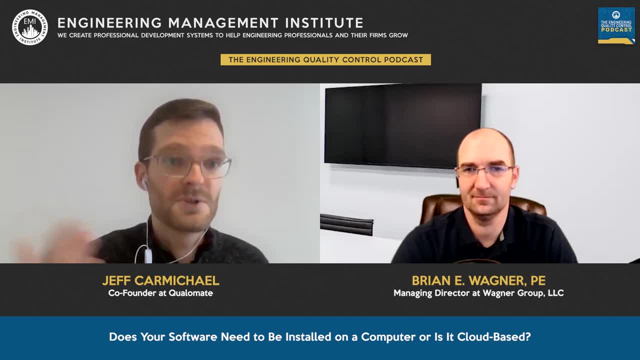 um, and they were building facebook at first and they just had so many users that they had to keep buying more and more servers and set them up and doing all that stuff. you don't have to do that anymore. it's just the click of a button and you've got all the power of of amazon's. 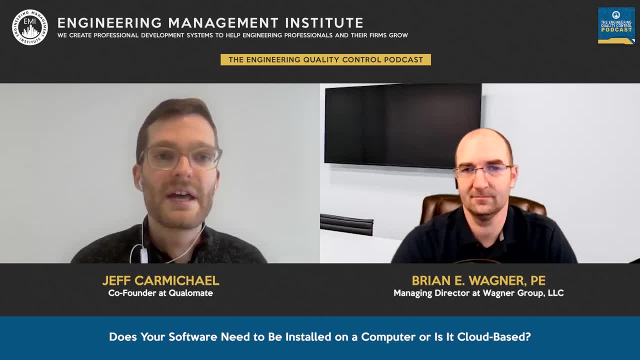 you know, global data centers, um, so it's really powerful and i think it's it's going to just become more prevalent in in every aspect of of our lives, um, but even, especially, um, not even civil engineer or not even software development, but but civil engineering itself, um, you know, if you, if you. 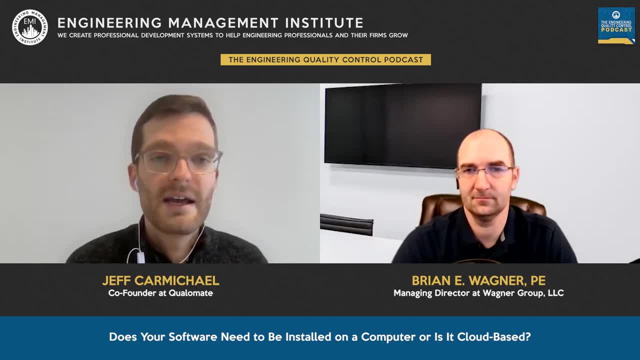 work in an office, like a lot of the consulting firms i worked at. uh, you know we had i have a server room that's, you know, locked and don't go in there. um, so that's the kind of like the kind of on-premises uh servers, um, which is kind of the opposite of cloud computing. um, so, a lot of. 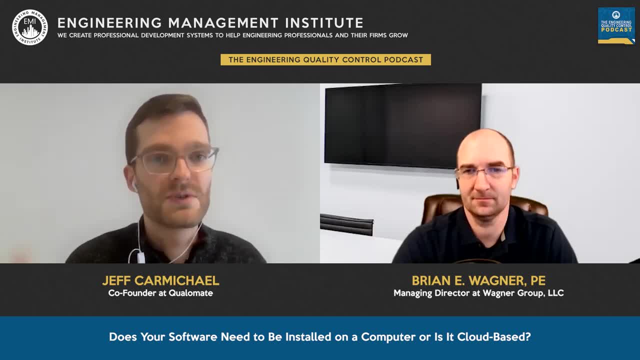 companies are sort of migrating from those those server rooms to to the cloud and that's providing so much value because you get access to, you know amazon's- just you know they've got thousands of people building all these cool tools that you can use and leverage in your, in your day-to-day. 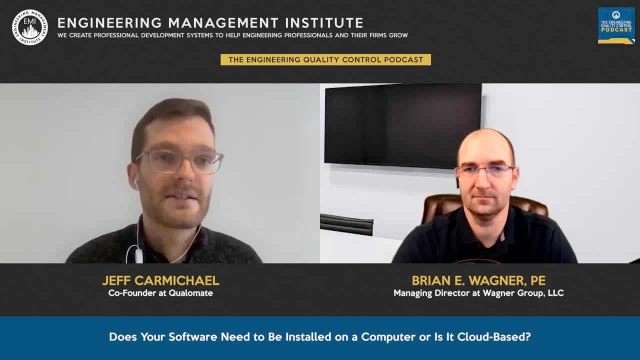 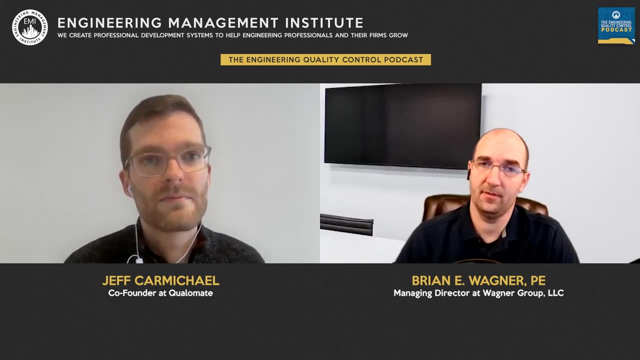 um, so yeah, i think that's going to make a huge, huge impact in, especially in the civil engineering and construction of, yeah, just kind of making all those processes better and centralizing the data and leveraging those. right now it's probably been accelerated a little bit with the hybrid work environment and the security of technology and the hacking and ransomware and 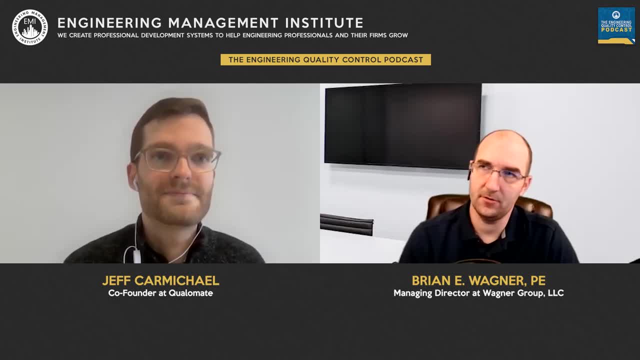 all those different things, so i can definitely see where you're coming from. so you mentioned that you didn't have a software development background per se, so you taught yourself anything for this? or like, what advice would you have for somebody that has an idea but really doesn't know what to do with it? or not trying to create competition for you, obviously, but 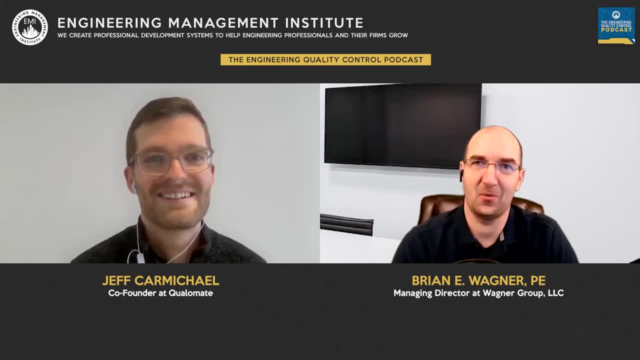 like if they have an idea that they think can make the workflow or work make their life better. what advice might you have for that in the similar scenario? yeah, i love, i love that question because it's it's there's so much potential for for people like civil engineers and just people. 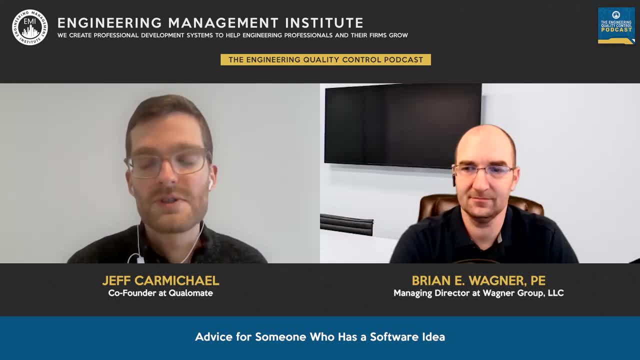 that aren't software developers. it's getting a lot easier for those sorts of things. so kind of the. i kind of started off on maybe two different paths that simultaneously that sort of merged into one. um, so first one is: is uh, learning how to, how apps work and that sort of thing. so kind of how i learned a lot of that was through. 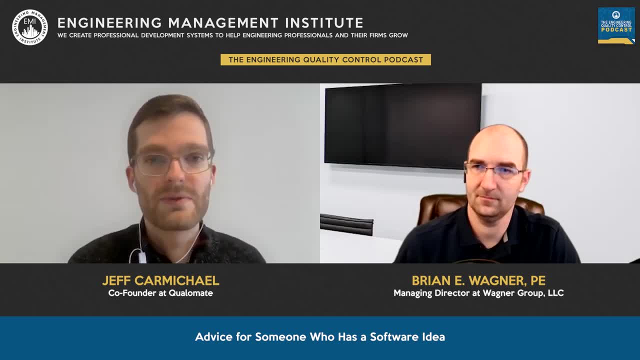 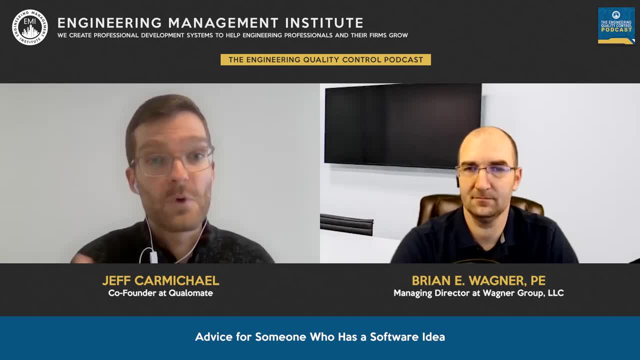 we were doing um for the, for the project, um, so we were, you know, pasting everything into a spreadsheet and it was sort of, it was kind of very just ad hoc, um. so i, you know, built a simple app in the matter of an afternoon, um that we could just type in, you know what day it was, and 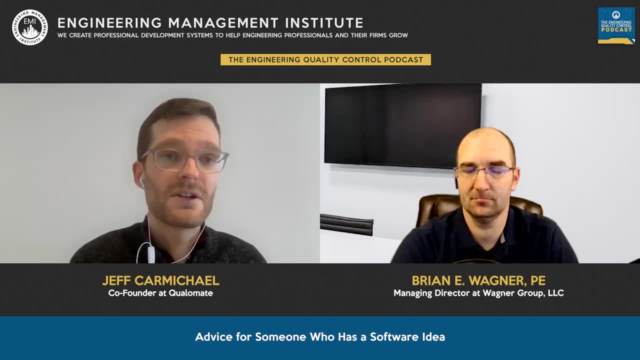 say where we needed the test and the information that the lab needed to know, and then it would send out an email uh to the, to the testing lab, um, and yeah, so that was, that was a great way to learn, like how how forms and databases kind of interact uh together, um, and then kind of on the 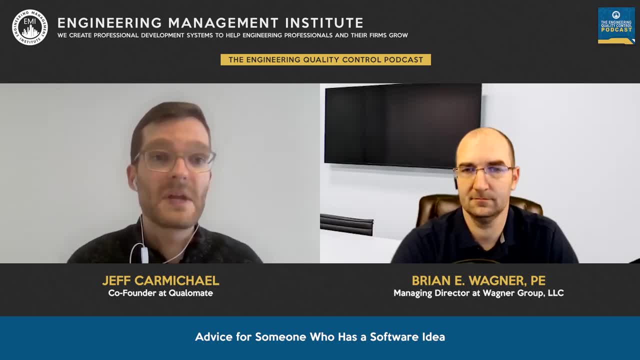 other side of the uh, software development. um, like i said, i was that part got started because I was interested in artificial intelligence, um, so just kind of started reading, reading about that and then wanted to kind of try it out. so it was brushing up on my, my python. 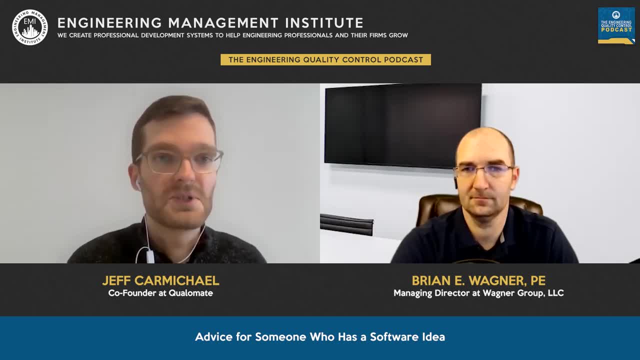 skills, uh, just trying out tiny little projects, uh, you know, simple, simple stuff, like you know a program that plays rock, paper scissors against you or something like that, and and then just slowly building up, uh, that, those skills, and you just kind of, um, you know, watch some youtube videos, uh, but most of it is just setting out a small project and then 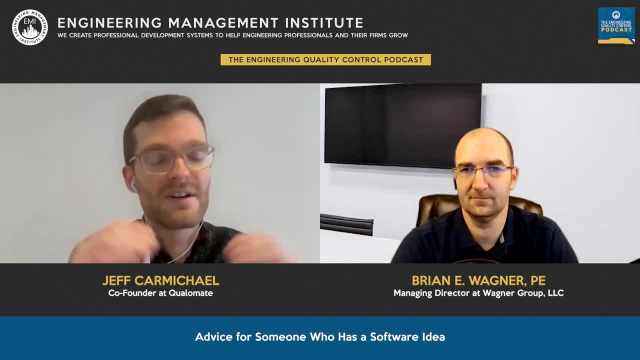 getting as far as you can and googling how, like, how do I do this little part, um, and then just that, just, really just steady practice on those sorts of things just builds up that knowledge and then you kind of um so combining the, that actual writing code, with the architecture of how apps. 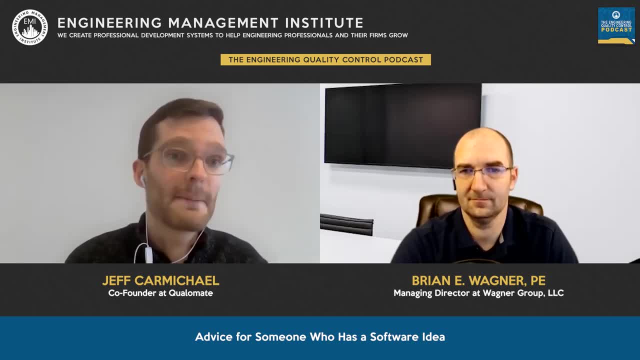 work. um. so, yeah, like things like uh, app sheet and power apps from with Microsoft, um, just kind of slowly, slowly building up that, that knowledge. um that you know it's not the same as I was to go to school for software engineering degree. um, there's lots of things that I I don't learned, yeah, um, but it's the best way to learn is just. 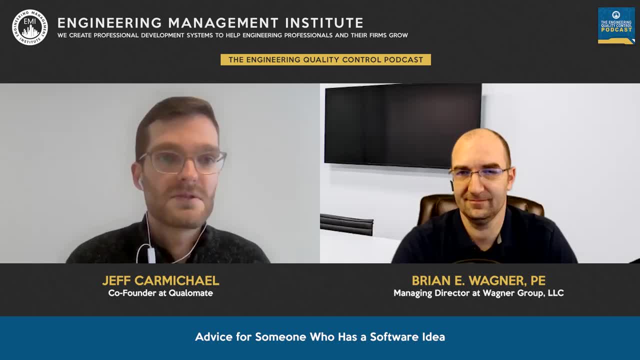 just getting started, um, and it's. you know I've got. you know may not be it's not going to win any um software design awards or anything like that, but you know it definitely works. it does exactly what it needs to do, um, and that's that's the important part, if you want to. 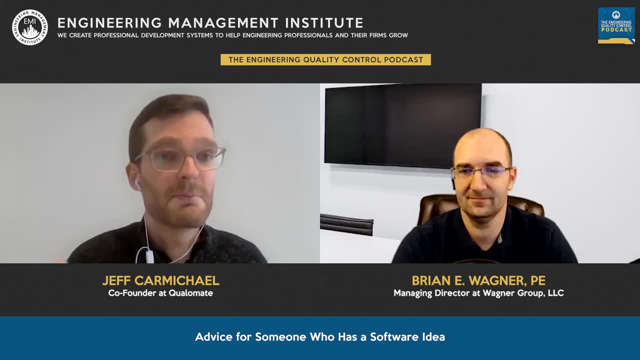 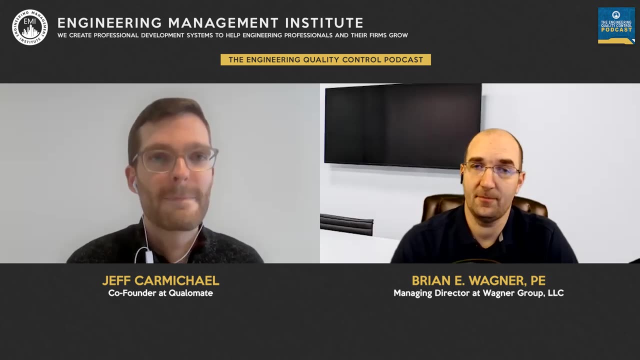 started on something. it's just building it and then if you need to make it a bit more efficient down the road, then then you can do that later, but you'll have time to do that. well, i you mentioned youtube and i feel like i learned- i've learned so much from just youtube and just searching. 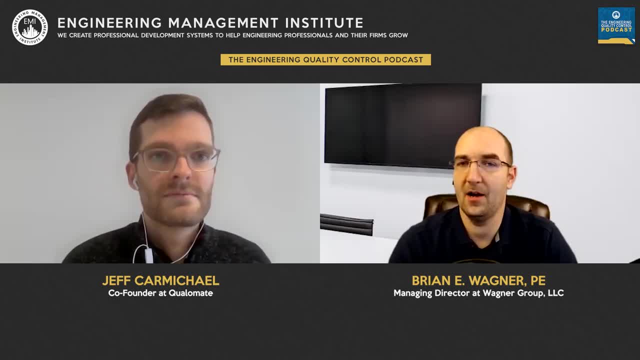 something and mine normally relates back to like excel, or i wanted to do this. how do i get it to do that? um, i've used microstation on a daily basis so it has the vba add-on coding stuff, so i've learned enough to be dangerous. i always try to comment enough in the background so that if 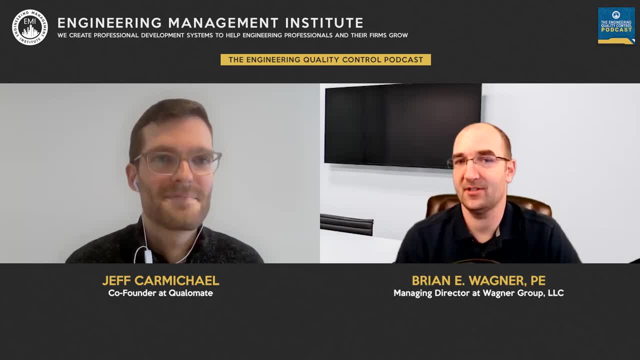 somebody actually followed me, they might actually be able to follow my thought process, but more than likely they would be lost and it probably follows no standards. but, like, use that trial and error, make it do what you need it to do. you make it happen, right? yep, yeah, and exactly like the comments, putting comments in your code. 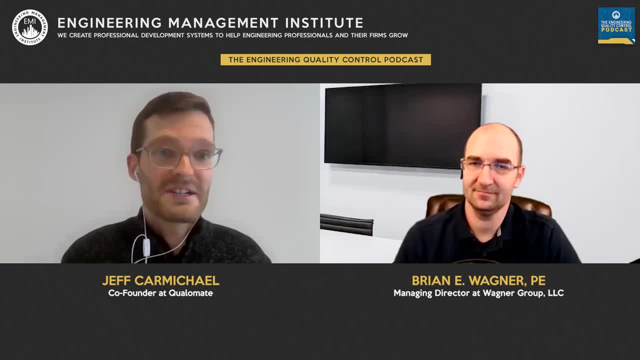 is probably one of the most important. quality control, maybe it's more of a quality assurance thing, um, for software. it's just having that documentation, um, so that somebody can can follow that process, and that's that that. that in itself is huge, the difference that, um you know. 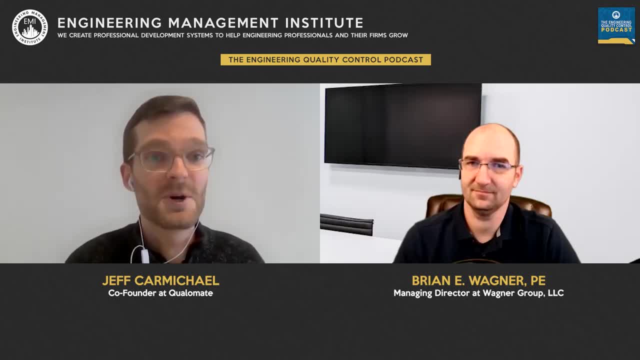 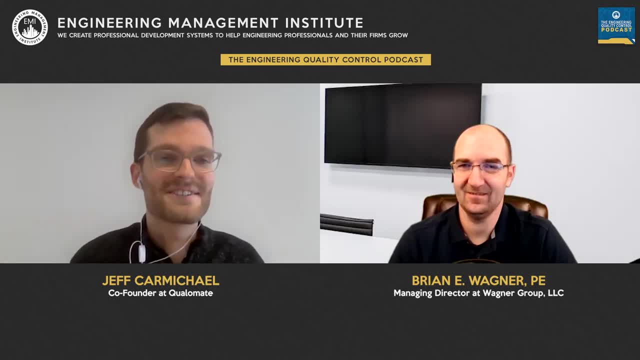 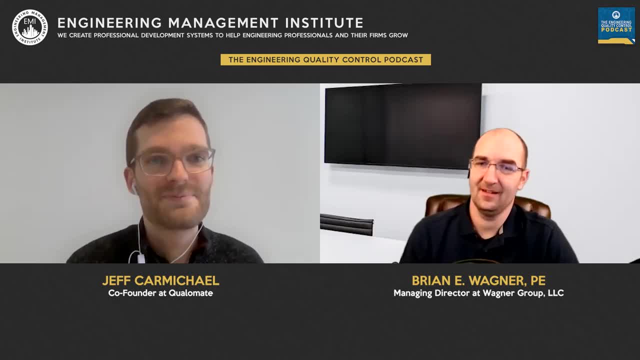 pretty early on and just make sure everything's well documented. yeah, and i think that's key to to the engineering mindset that so many people have is just like explain yourself or answer, have those questions answered because there's so many what-ifs and engineers in my experience have. 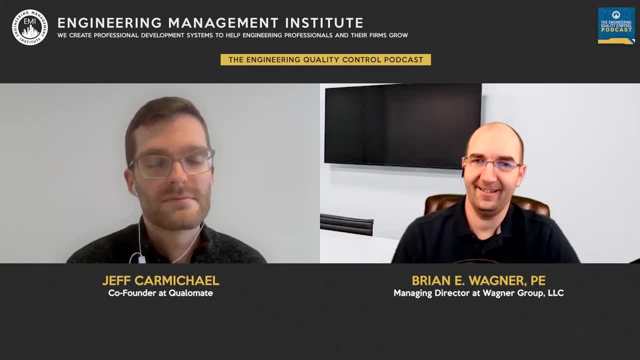 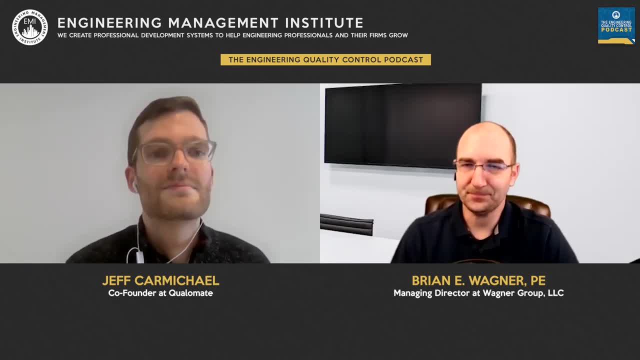 to how they want to finish something. do you know? i'm saying definitely so i want to be courteous of your time, don't want to take up too much of it, and because i know you're busy. but, um, we do like to include a segment in every show- we call it the power of experience segment- where we ask you just 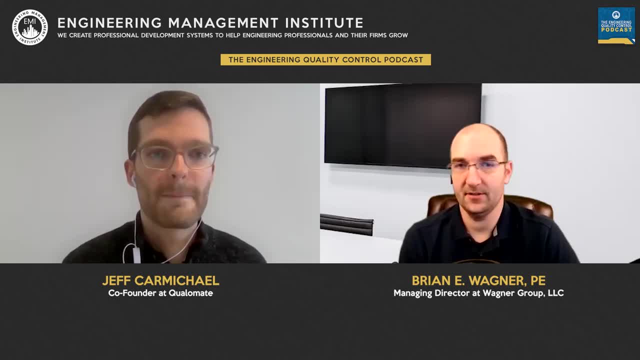 to offer a piece of advice to the listeners, whether it's in your experience, in what we've talked about, some other engineering experience or just life in general. yeah, yeah. so i think something that's that's worked out well for me and i've kind of taken 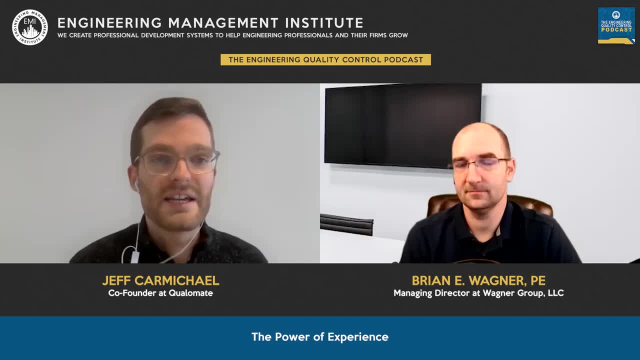 advantage of throughout my career is, um, you know, saying yes to, to opportunities that that come up, that might be. you know you're not really comfortable with um. for example, you know when i first got started- uh, actually, when i was still in university- over the summers i was given the 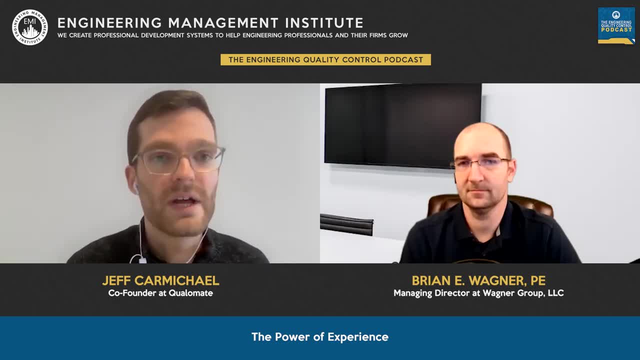 opportunity to to go work in in northern canada and fly in uh towns, um, so that was. so i said yes to that, um kind of spirit of adventure sort of thing and see what happens um. but yeah, worked out really good. we had. i had a ton of fun, got a ton of ton of experience um and and different sorts. 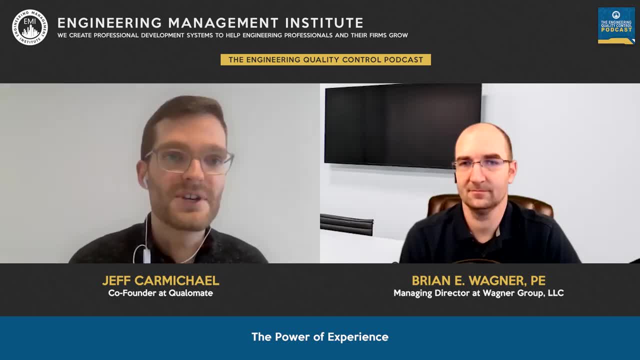 of things. like you know, it's different types of challenges and different types of problems that you have to solve when you can't. uh, you know the next town is six hours drive away, sort of thing like that. so that was really cool and, um, uh, kind of same thing happened. 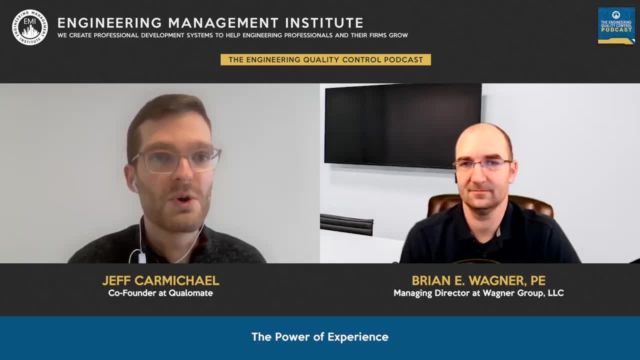 to move to new zealand, sort of on a whim, um, with no connections in the country or anything like that. um, obviously you know you want to make calculated risks. um, uh, don't just do everything. um, but new zealand was a country that had, you know, big engineering skill shortages, so there's. 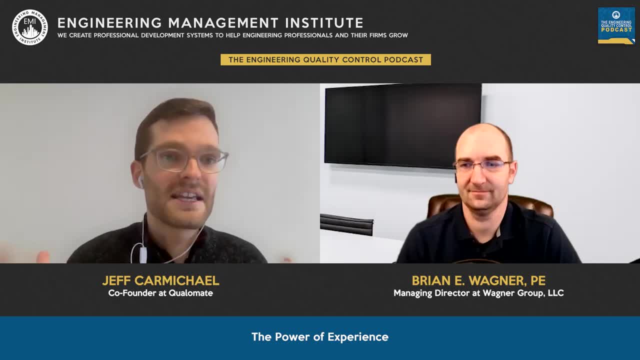 lots of jobs and that sort of thing. so, yeah, just kind of take, take the leap on something, um, maybe it's travel, uh, maybe it's, you know, learning, software development, um, it could. yeah, it could be all kinds of things, but just if you have an opportunity that you're kind of hesitant on. 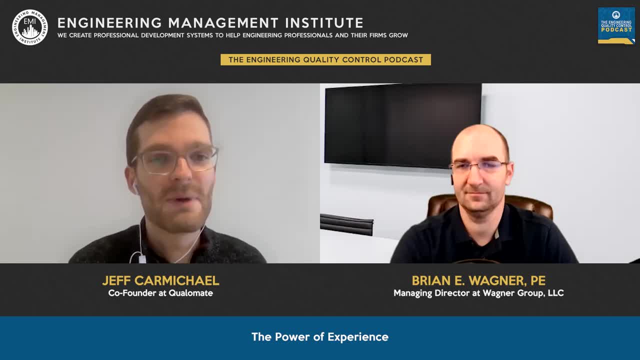 um, i, if you're you know, think about it for a while, but that's it, that's it. jump right in. no, i think it's great advice. uh, yeah, i'm thinking about things that i've said yes to over the years and things that i've said no to that. i don't say i have regrets, but at the same, 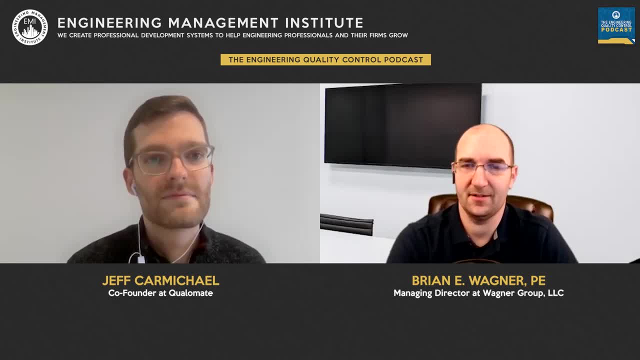 time, i might have been able to get some valuable information or insight out of certain things that i said no to and that's long since passed for me. um, i just want to give you the chance so you do have a software that is available for for people to use right now. yep, uh, we're doing beta testing for the next, uh, probably two or 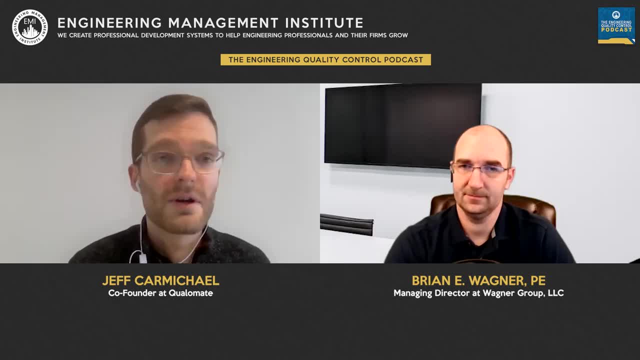 three weeks, but then we've got some projects coming online in, uh, early to mid-february, um, so yeah, if you're interested, um, we can get you set up next couple weeks. so, like what type of if you were to sell this to somebody or offer this? 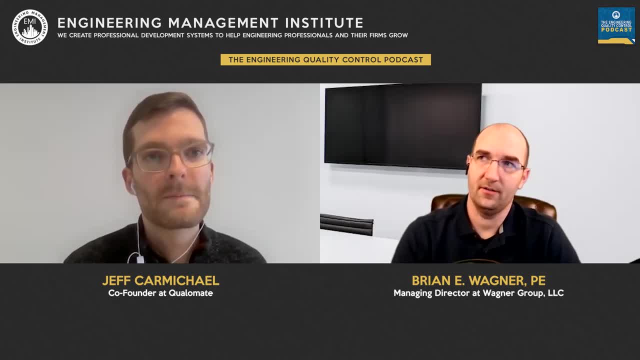 to somebody like: what, what would be your target if there's a listener on here right now like: who are you talking to? as far as that, you could help today. right now we're focusing on those um infrastructure, civil infrastructure projects, so um roads and our first clients- yeah, our first. 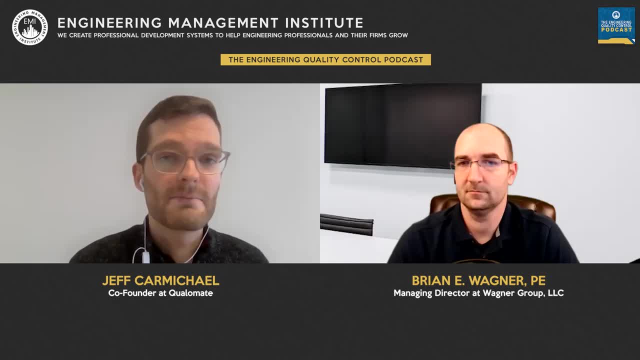 two clients are going to be a big road widening project and, uh, commuter project, um, so that's sort of our bread and butter at the moment but, um, a little bit farther down the road we'll be looking into supporting um, uh, you know, commercial and uh, any any of the bigger.